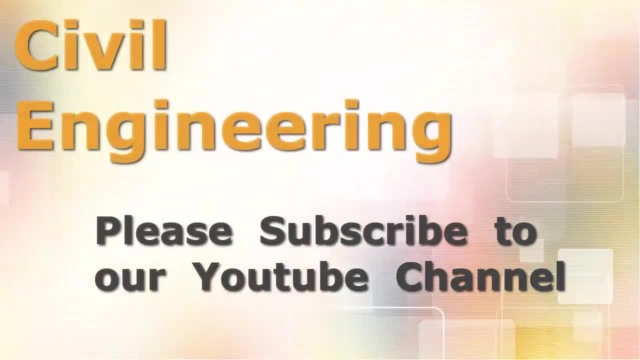 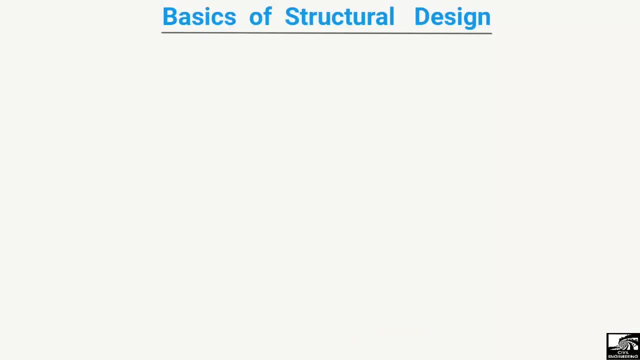 Hello guys, welcome back to E7 Engineering YouTube channel. Please subscribe our channel for daily E7 Engineering videos. In today's lecture we are going to discuss the basics of structural design. So here are some basics, from the plan of a structure till to the design. 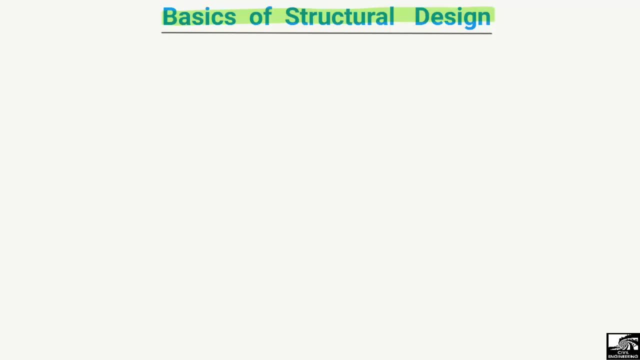 and detailing of the reinforcement in a structure. So the first step in the structure design is the structural plan. This is the first step and we decide this step with the architecture, that how we can build our structure element. So this is the structural plan for any kind. 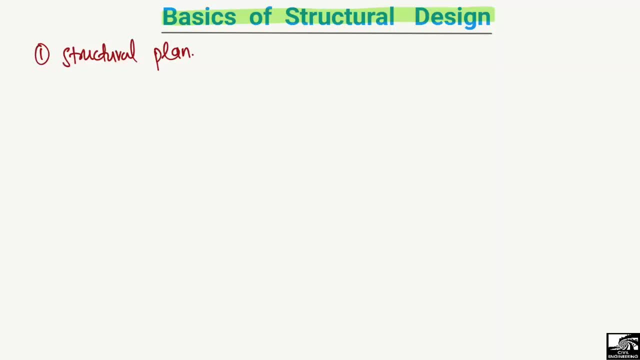 of building or structure you want to design. So the next step comes with the type of a structure. It means Now, which kind of structure are you bringing on the structure, What type you want to build? either you want to build it with a concrete only. I mean the. 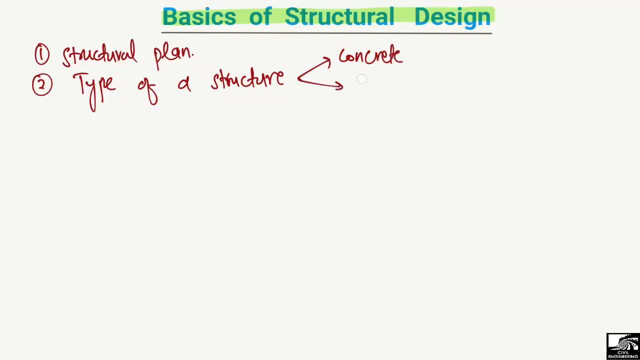 reinforced concrete structure, or you want to build the structure with a steel, just like completely made with steel structure, or it is a kind of a wood structure, so it may be another kind of a structure. so the second step is to decide about the type of a structure. the third one is: is the assumed member size? 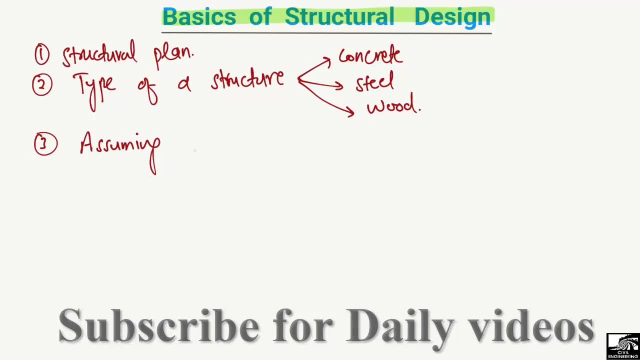 or assuming a member size. now, after decide, after deciding that we want to- for example, we want to design or take the structure which is made up of the RC concrete or the reinforced concrete- now the next step will to decide the member size. for example, it includes that what would be the size of the beam? what would 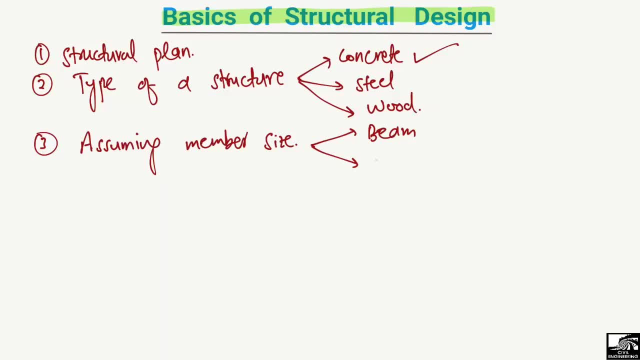 be the size of the column. so this comes under the design criteria- column, for example- and we have to know, we have to design or assume our member here- for example, the beam dimensions. we have to take it on the first step. we have to assume this dimension, for example, the width of the beam or the depth of the. 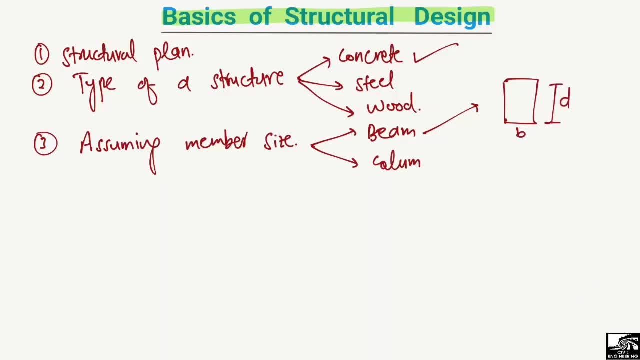 beam and according to this we have to design our member. so the third step includes the assuming the member size and designing it accordingly. it also includes the column. we have to take certain dimension of the column, which consists of its� and the depth of the column, and accordingly applying the friend on this. 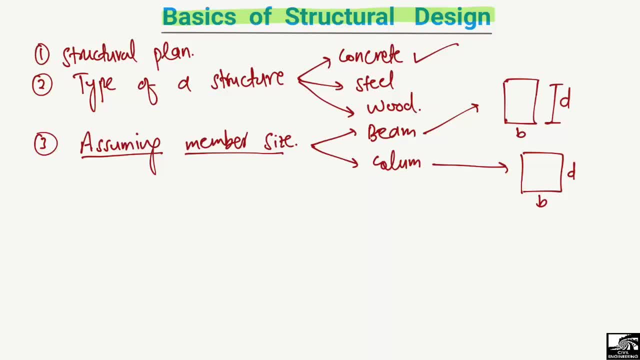 and then later on to provide the reinforcement for these structure members. but the first steps are, we can say: the third step here in the design comes out to be the assuming the member size. the fourth one comes out to be the applying loads on this structure members, applying laws. now, what is mean by load? 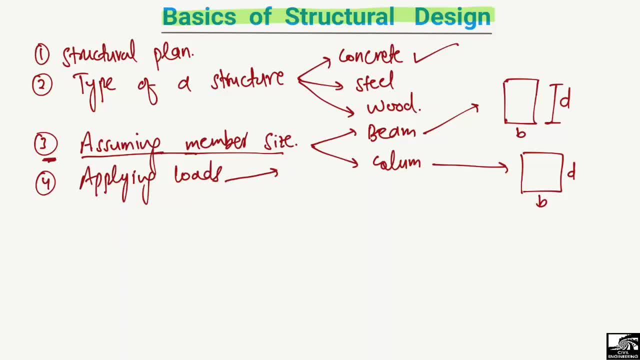 because we know that the structure may be not alsoност for the project. the location- and therefore I have two mine columns- will have self weight, or we can say it will have dead load. it will also carry some live load, depends on how you want to design. for example, there are: 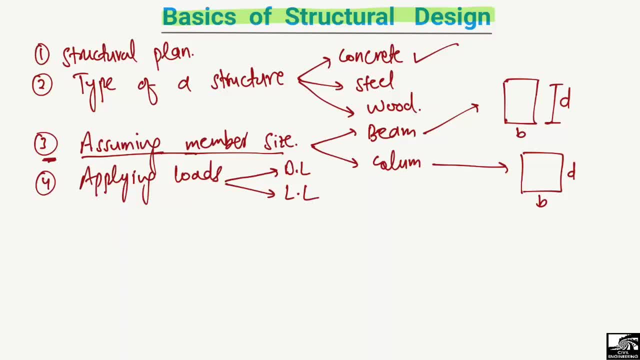 different standards which provide the different loads for your building element, so you can also put the snow load on your building element depending on where is your building. for example, if it's in snowy region, then you have to consider the snow load, and if it's a very tall building, more than 80 floors. 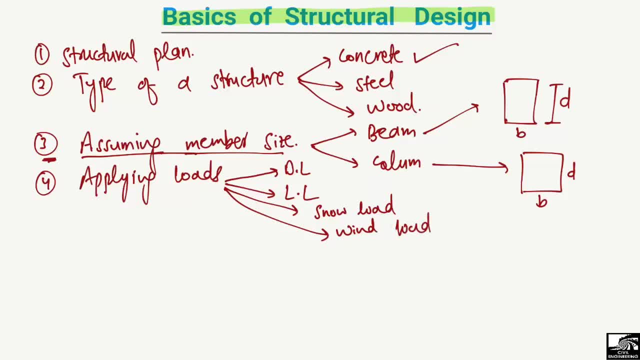 or something like this. then you have to also consider the wind load acting on this building. so we have different kinds of load in which we applied these loads on our building and also we have to combine these loads or we can say the combination of load should be applied to the structure members. combination of: 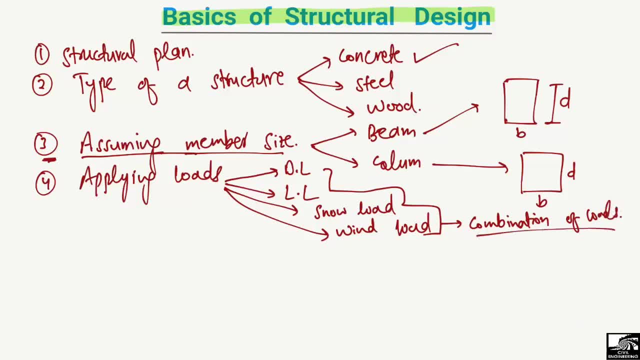 loads. there are different combinations of loads in different cores. for example, you. According to the American, it states that 1.D dead load plus 1.6 live load. According to the Europe, which I remember, it's 1.35 dead load plus 1.5 live load. 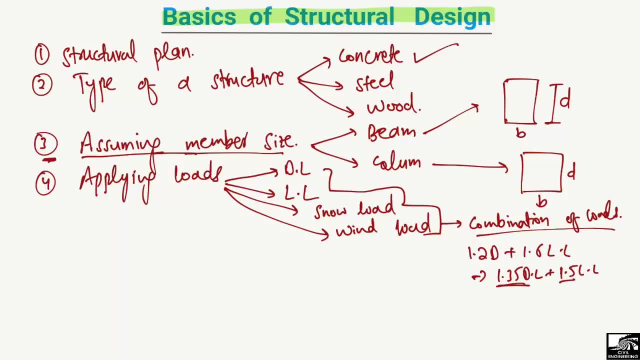 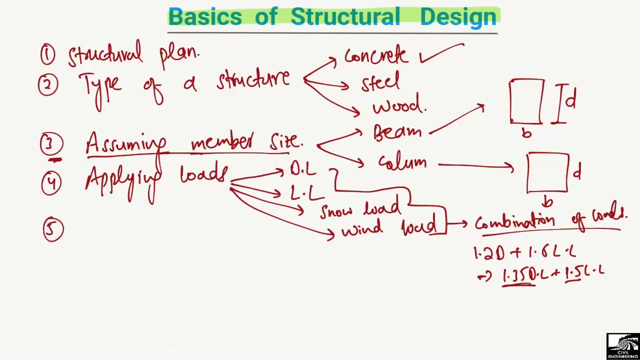 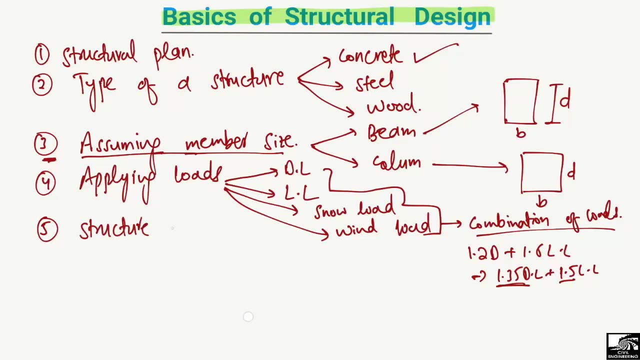 You have to multiply it with a factor in order to increase the load demand on the structure member. So the fourth step is applying the load on your structure, Now coming with the fifth step. the fifth step is about the structure analysis. Now, after applying the loads on the member, you can do analysis of these structure members. 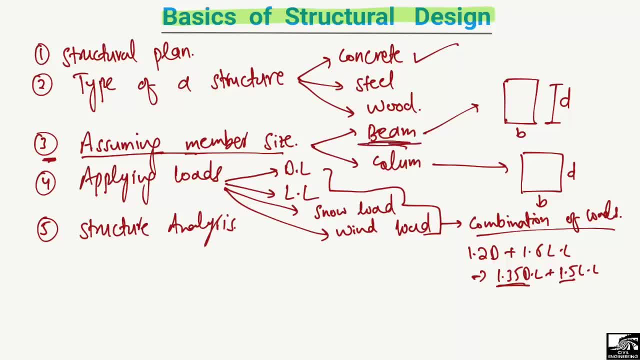 So you have beam. you took the assumption in the dimension of the beam and then you applied the load on the beams and then you have to do the structure analysis. Structure analysis now includes the shear analysis. How much is the shear forces acting on your beam? 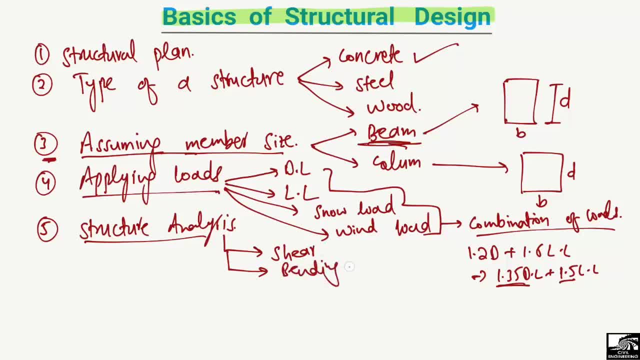 What about the bending moment, The maximum bending moment coming on your beam structure, on your beam element? Also, for torsion stresses acting on your beam, there are different, various analysis that we should carried out in the structure analysis. So after getting all of these analysis- shear bending moment or torsion, for example- then 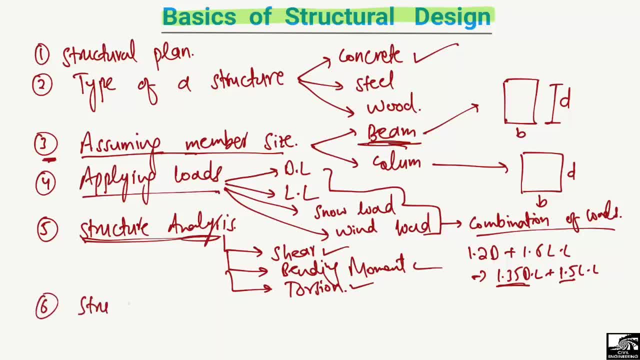 we are going to structural design. The next step will be the structural design. In this step we have to design our beam element And it includes the structure. The structure element is the area of the reinforcement, So it is related to the area of the reinforcement. 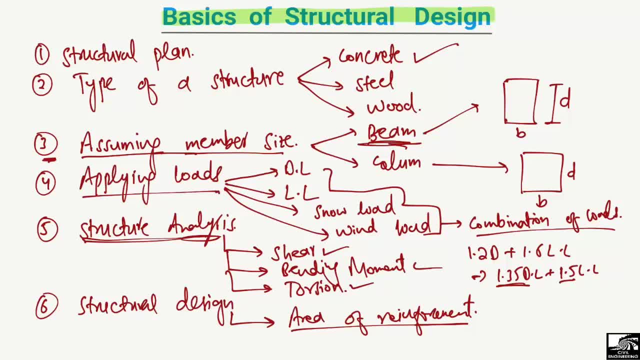 That how much area is to be provided for your structure member in order to take the load, You applied the load on your members here and then you do analysis that how much shear force or bending moment are coming, and then you according to the bending moments coming. 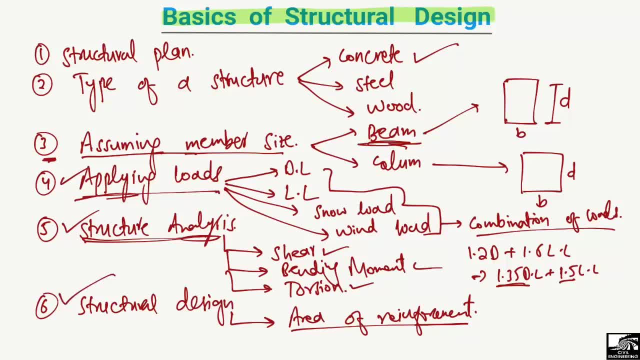 on your beam or shear forces. you provide the design for these members And from the design You took the area of the reinforcement, That how much area of the reinforcement should be provided in order to take the applied load? So 6 is the structural analysis, structural design. 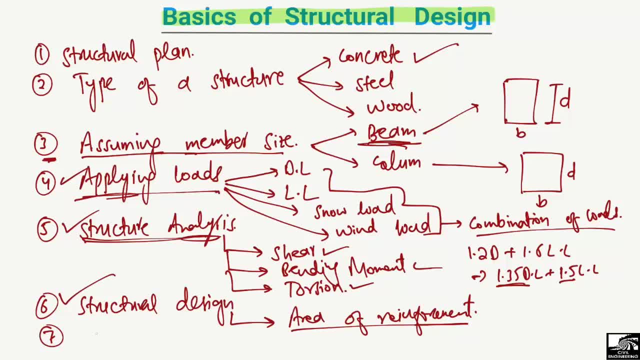 Now the 7th step. 7th step comes with the checking for allowable limits. After your design is satisfied, for example, the area of reinforcement you provide, satisfied the load, Then you have to check the check for allowable limits. Okay, 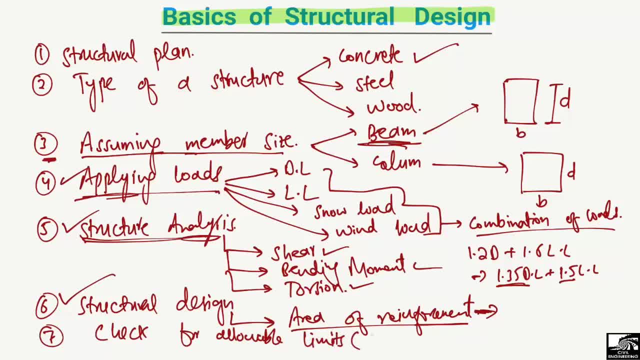 Okay, Okay, First check here, And this is mostly for serviceability analysis. or we can say for example here deformation or deflection, And it should be okay, Otherwise you have to repeat the whole steps. So the 7th one is for the serviceability analysis and we have to check for allowable. 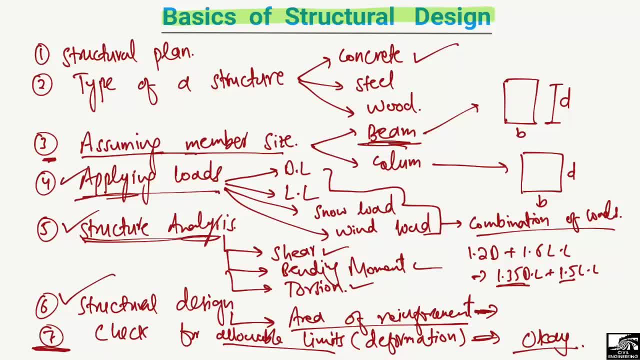 limits. It means that there are different codes which provide different limits for your deflection of the members, for the beams columns, For example. so this is my beam with the length of L, so we need to find out its maximum deflection. for example, it deflects like this and this is a maximum deflection. 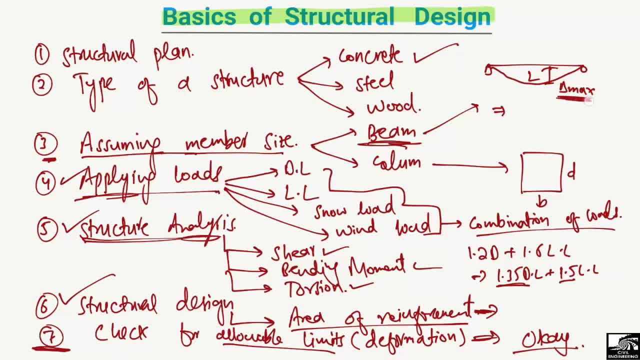 here Delta maximum. so you to verify this maximum, this maximum deflection of the beam, and it should not be less, it should not be greater than the maximum deflection provided by different codes. so this is comes under the category of the serviceability. so we should consider this serviceability analysis also in our 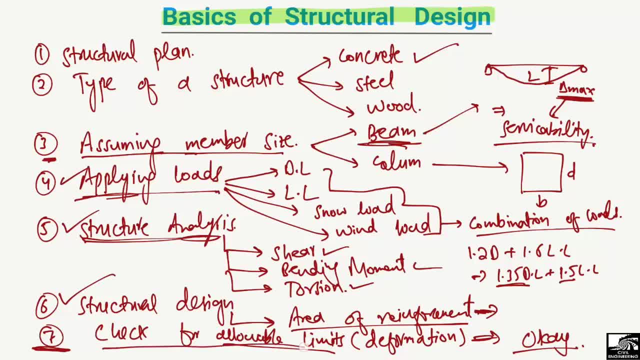 design. and this is the last step. check for the allowable limits. either it is greater than the one which provided by code or less. if it is greater, then you must have to redesign the whole steps, for example, from assuming the beam and then applying the load, structure analysis and then structural design. 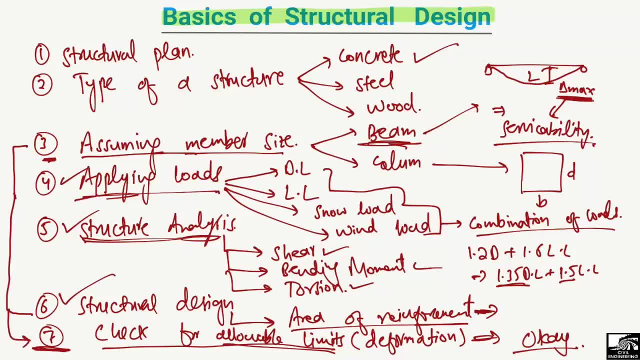 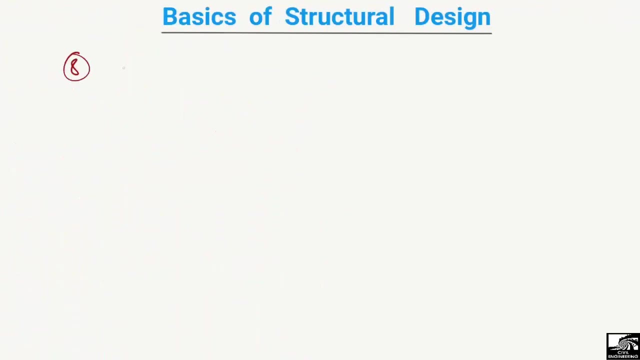 again and then again checking for the allowable limits. so if it's not satisfied, then you to go again, up and again down until it satisfy the serviceability analysis criteria. so hope you guys understand. and the last step, of course, the last step is missing here, so I can write it here. number eight step is about the detailing. 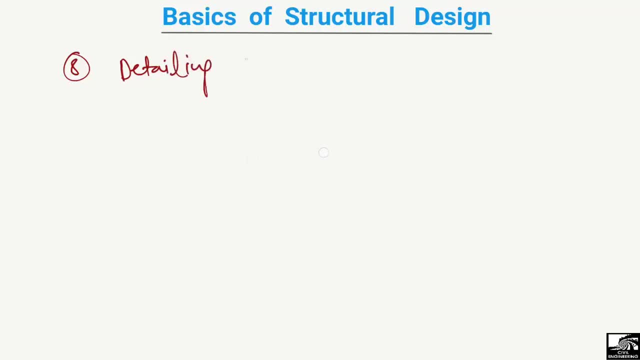 of the reinforced members, detailing, and this increase the ductility of your structural members. ductility, so, by detailing, means that the reinforcement should be provided in certain region in order to increase the ductility of the structural members, for example, if this is my, for example, if this is my beam, so, and this is also, 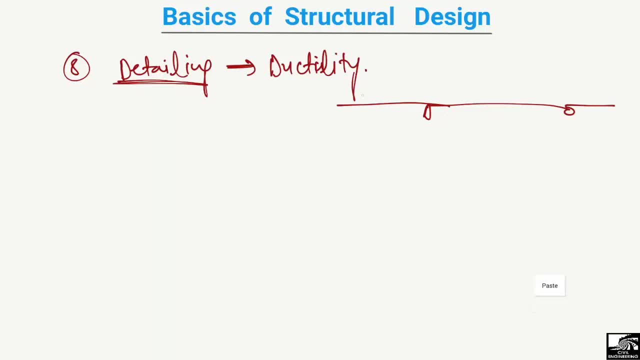 going in this both direction. so if this is a load acting on the beam and there is a deformation at the bending stresses, like in this way, and then again like in this way, so we have maximum bending moment in this mid region, maximum bending moment, positive bending moment. so we cannot provide. 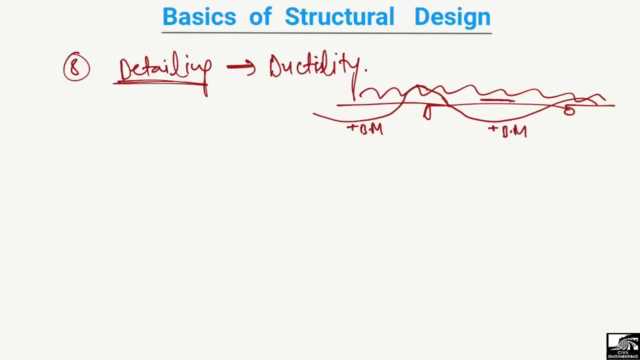 overlapping of the bars here at those region also at those region. so we can only overlap the bars here in the support region. also for columns there are different detailing rules which we should consider in our structure, members, in order to increase the ductility of the member and also to do it according.